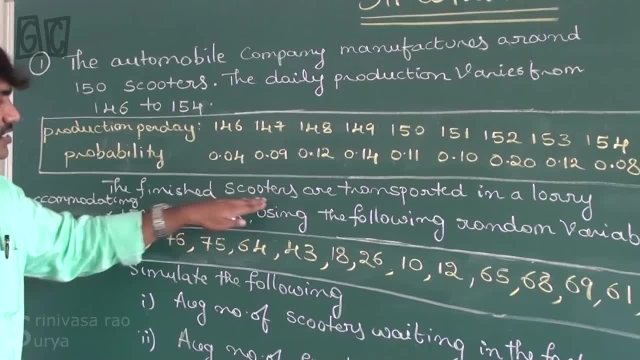 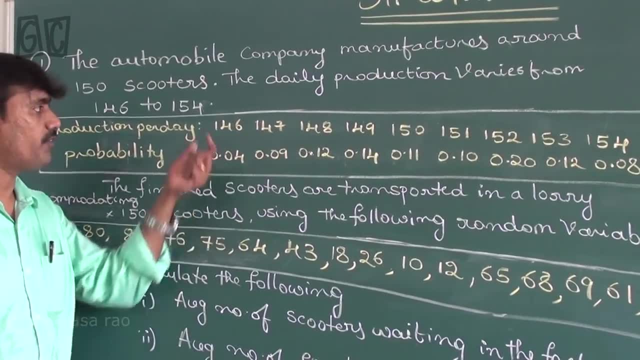 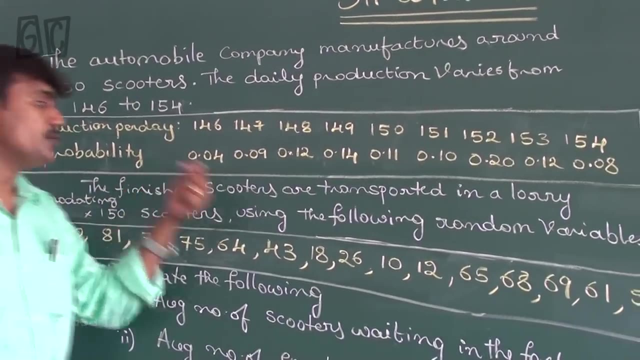 like this: And the next is the finishing scooters are transported in a large number of lorries The capacity of 150 scooters. So the finished scooters we are going to transport in a lorry. The capacity of the lorry is 150 scooters. Using the following random numbers: 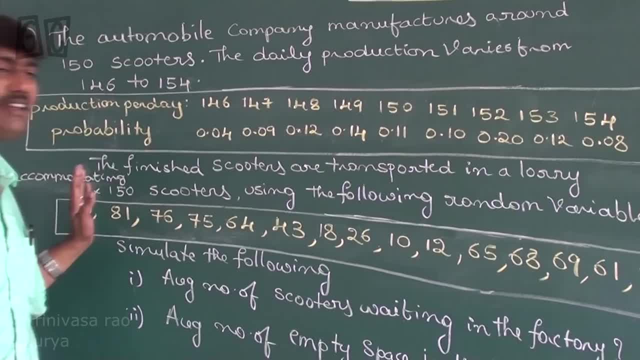 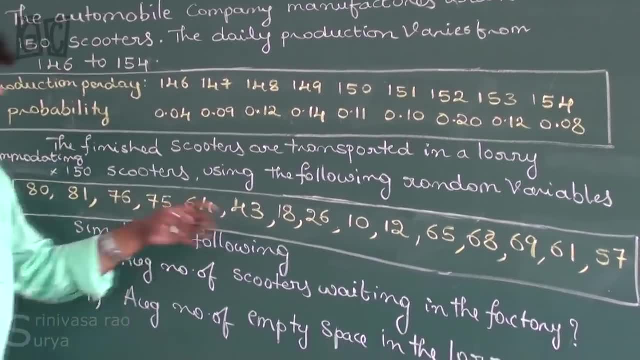 so we have 10 random numbers, we have 15 random numbers, With the help of this information, what we have to find? so we have to simulate the following: that is average number of scooters waiting in the factory. we have to find out. And the next one is average number of empty. 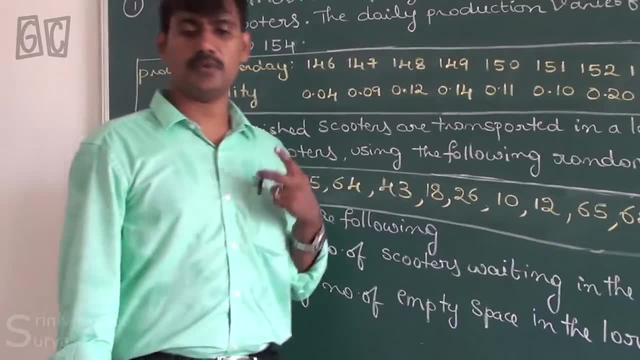 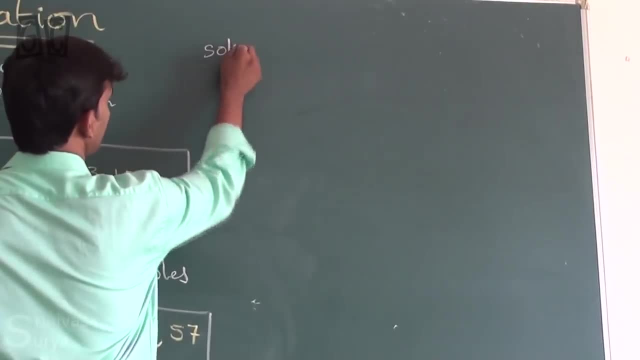 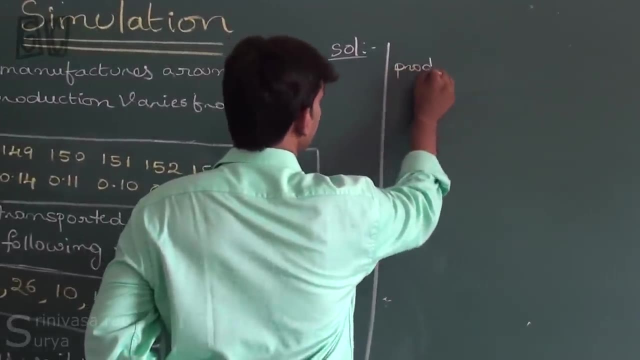 spaces in the lorry. So for this we are going to represent only two simulation tables. So the first table is our spots. So that is first we have to construct a table for the random numbers, So the given data we have, production per day. The production per day is given And 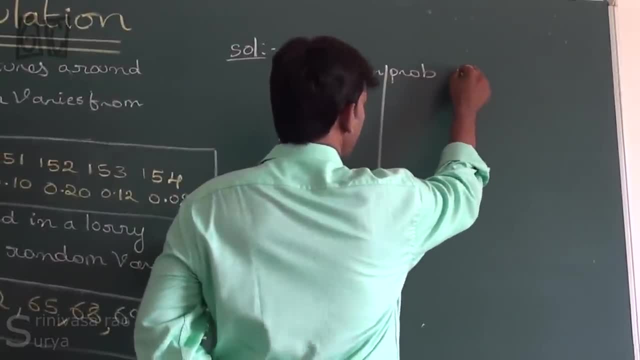 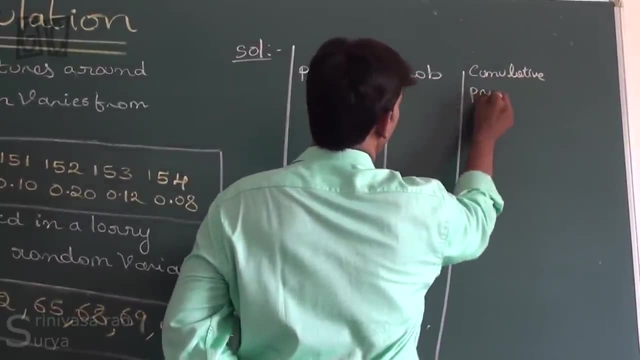 the next one is: the probability is given. After this, we have to calculate the cumulative probability. The cumulative probability we are going to calculate. So the cumulative probability, we are going to find out And the last one we have, we have to find out. 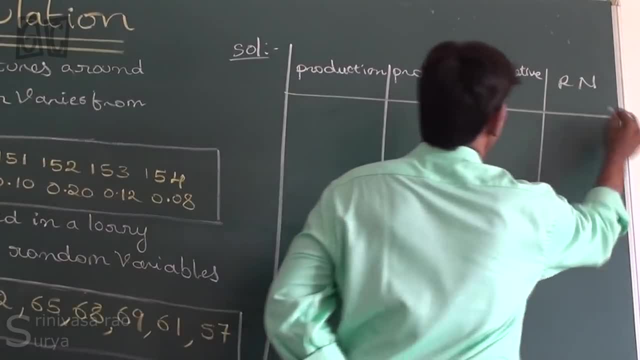 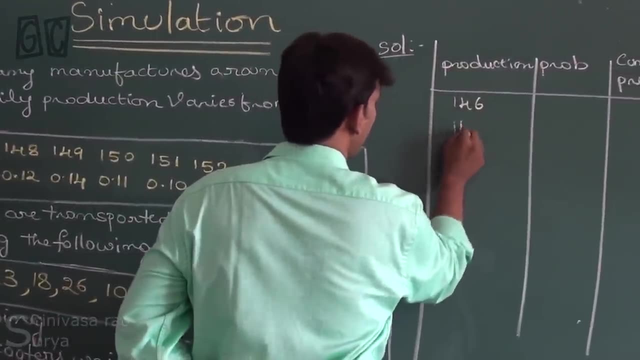 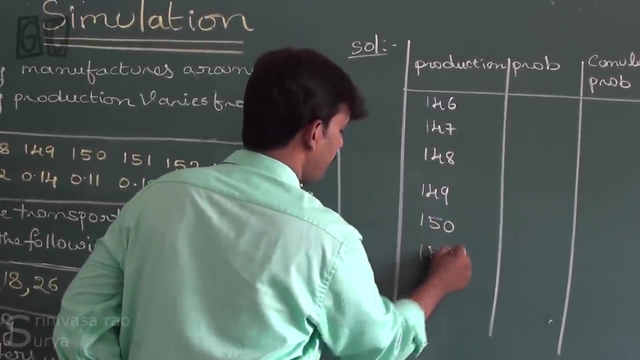 our random numbers. So these are the four columns we have to find out in the first. So the production per day is obviously 146, 147,, 148, 149,, 150,, 151, 152,, 153 and 154. 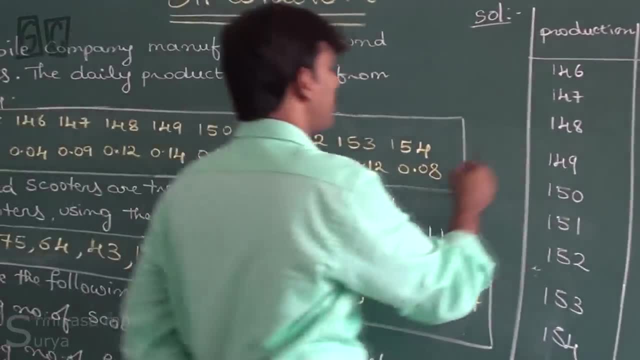 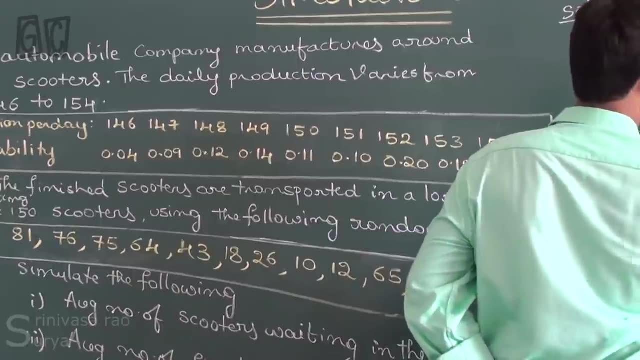 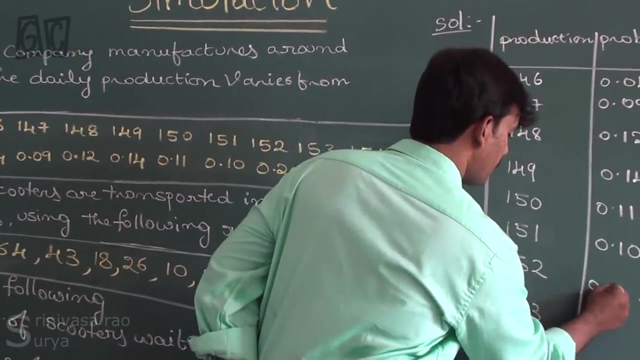 These are the given information. The probability we have given is 0.04, 0.09,, 0.12,, 0.14, 0.11,, 0.10,, 0.20,, 0.12 and again. 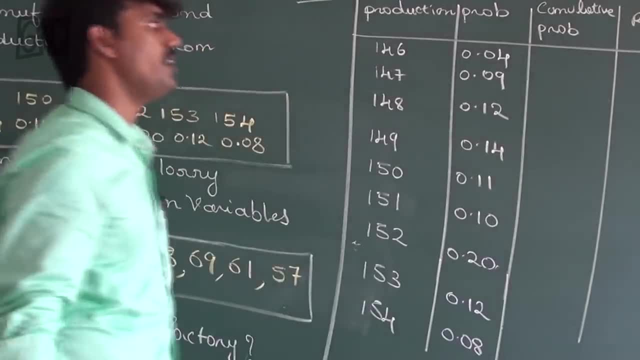 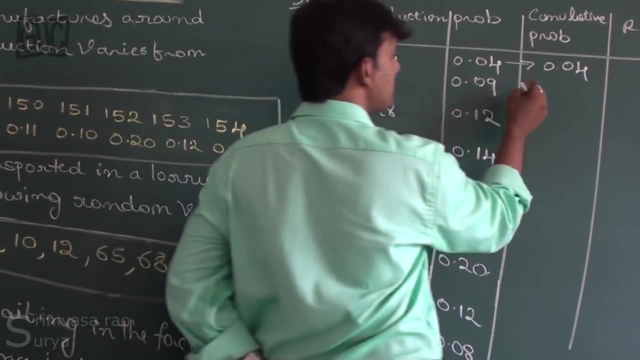 0.08.. Now we have to find out the cumulative probability. The first we have to find out is 0.04.. 0.04.. So 0.04.. 0.04.. 0.09.. 0.13.. 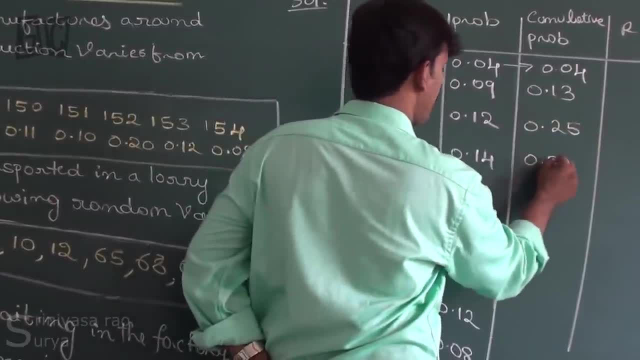 0.25.. 0.39.. This is 0.50., 0.60., 0.80. 0.92. And this is 100. 0.00.. This is the construction of the cumulative probability. 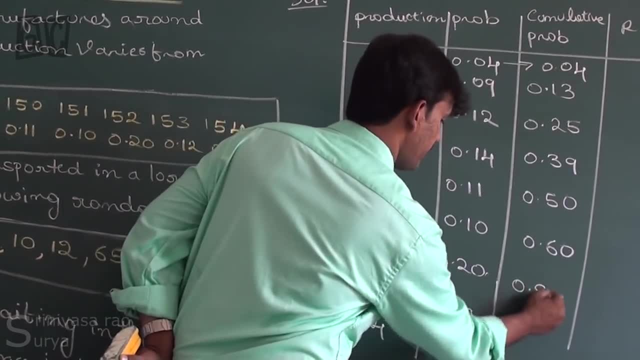 After that the random number stays, So 0, so that is 0.04.. Now we have to find out the cumulative probability, So 0.04.. 0.09.. 0.10.. 0.10., 0.10.. 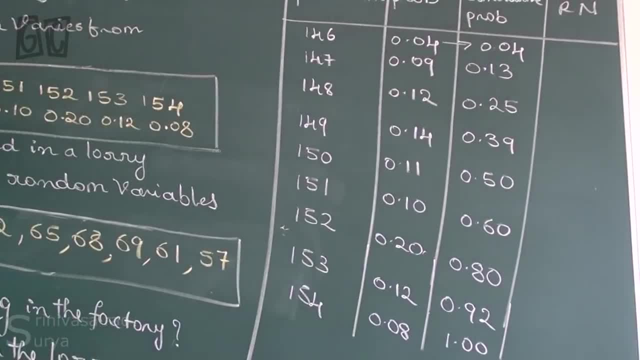 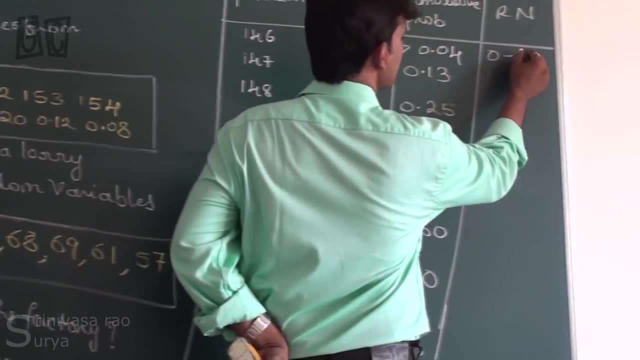 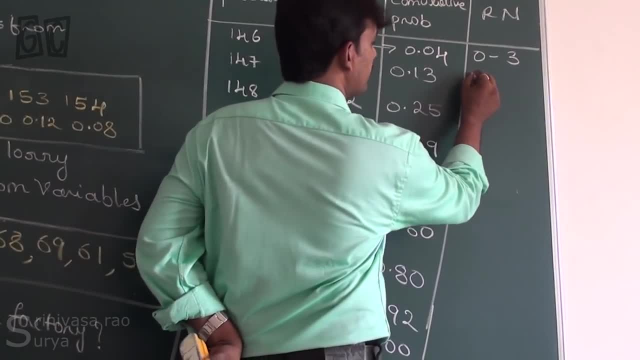 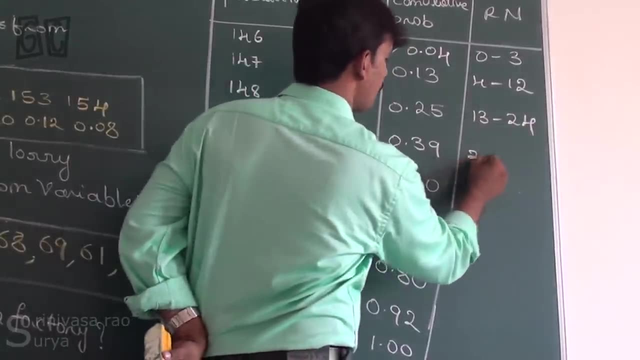 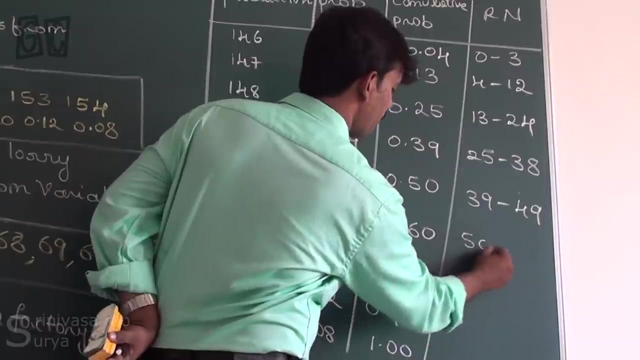 0.10.. 0.10.. Then come 0 to 3.. Ñ, That is again 4 to 12.. 30 to 24.. 25 to 38.. 39 to 49.. 50 to 59.. 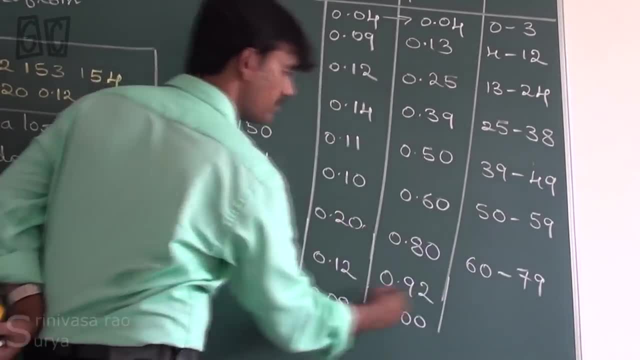 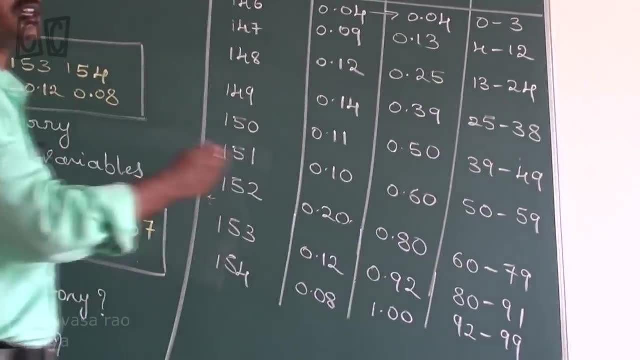 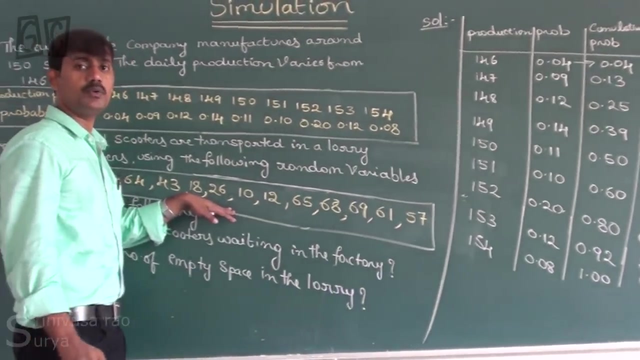 60 to 79,, just one less. 80 to 91. and 90 to 95. So these are about random numbers range. After that, with the help of these random numbers, we are going to check and we are going to find the average number of quotas waiting. 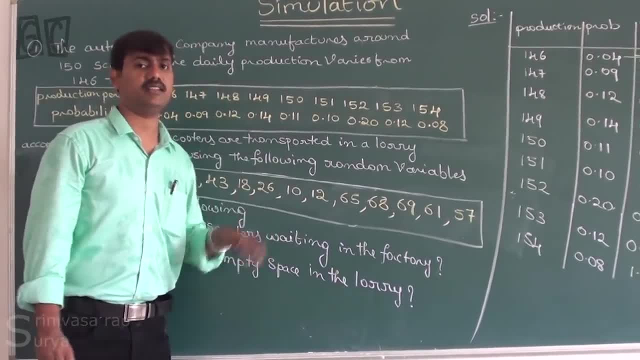 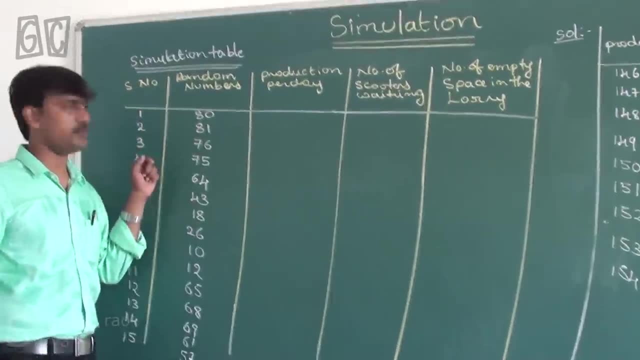 in the factory and the number of empty spaces in the factory. The next table is as follows: Okay, guys, so the next step for you is the simulation table. So we have a 50 in the ceiling, the quotas and they are in the cushion itself. We have a random numbers like 80,. 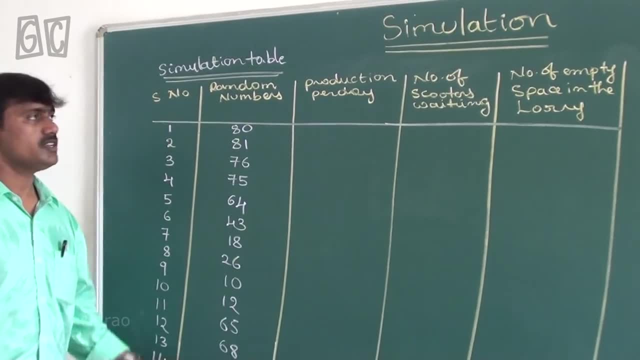 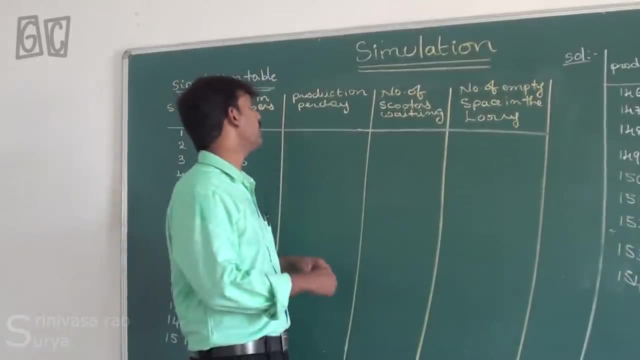 81,, 76,, 75 and 64 up to 57. So we have to find the average number of quotas waiting and the empty spaces in the lorry, and we have to find out those two conditions. So here we go. So this table comes with 4 columns. 1st one is the given random numbers i have. 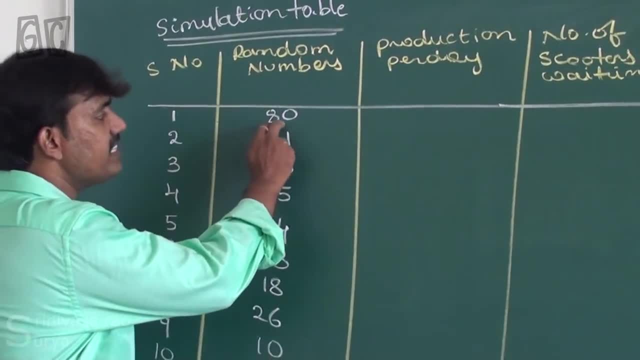 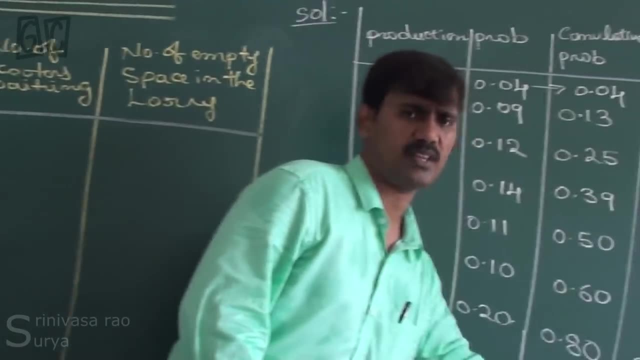 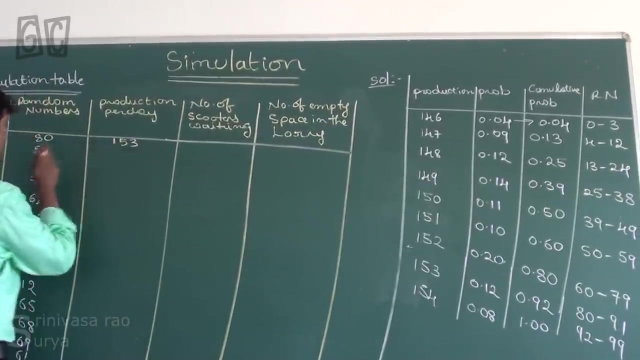 copied it here. all the random numbers: production per day: 80 is the random number, So that we have to check out that we will get stable. 80 is nice, So production per day is 150.. So production is 153.. So here we go, That is 153.. For 81: 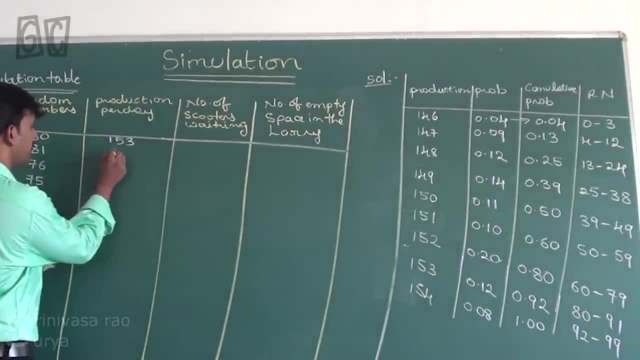 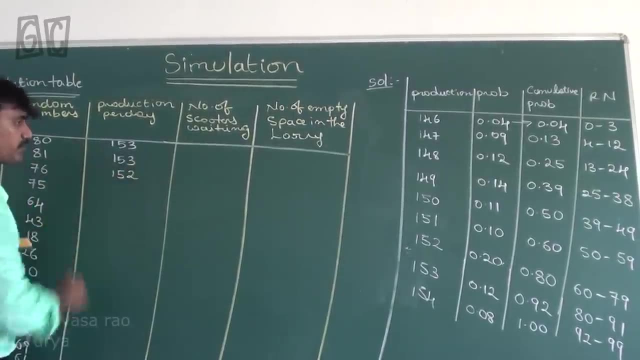 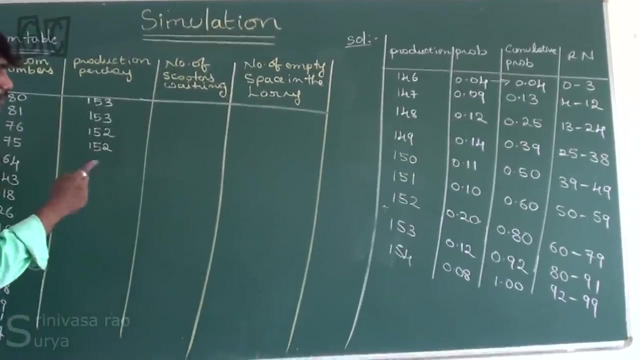 also lies between 80 and 91. Again, the production is 153.. Here we go. The 76 lies between- again 152, I guess 75 again 152.. So you have to check the interval over there- 64.. 64 means 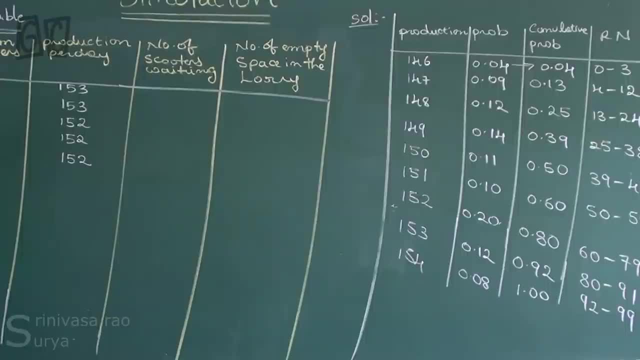 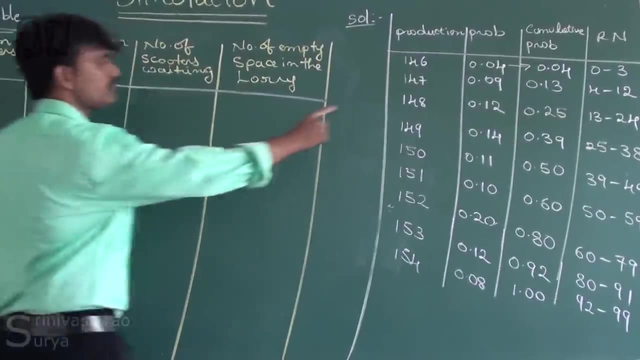 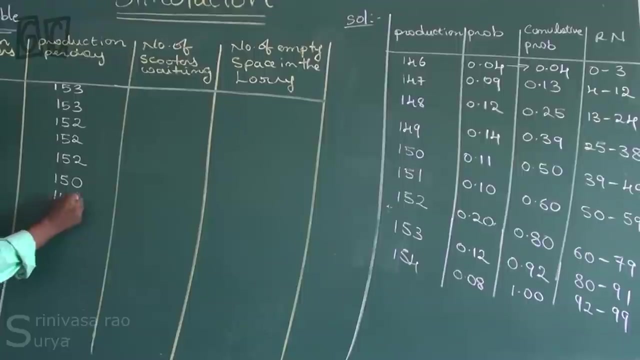 again 152.. 43.. 43 lies between 39 and 49.. The production per day is 150.. 18.. 18 means this one: 13 to 21.. That is the 80.. The line is 148.. 26.. 26 is the production per day. 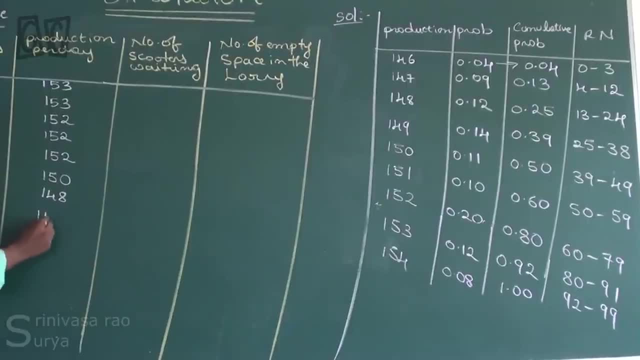 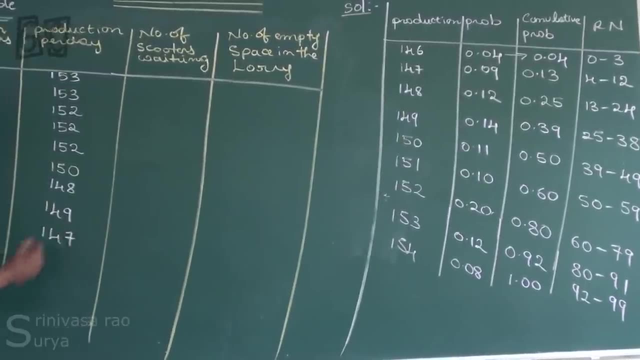 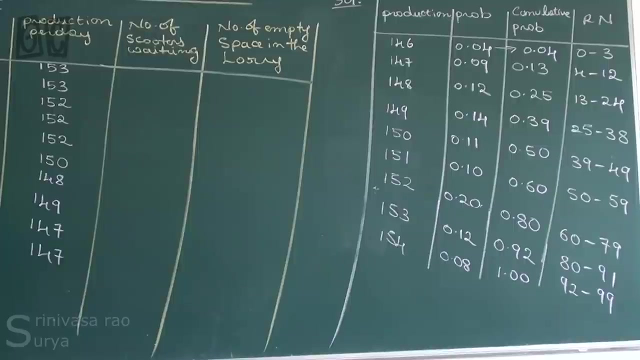 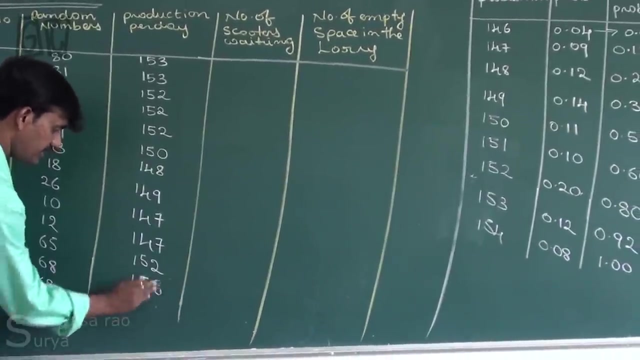 26 lies between 25 and 38.. That is 149.. 10 lies between 4 and 12.. That is 147.. 12 lies between again 147.. 65 lies between 60 to 79.. That is 152.. 68, again 152.. 69, again 152. Again. 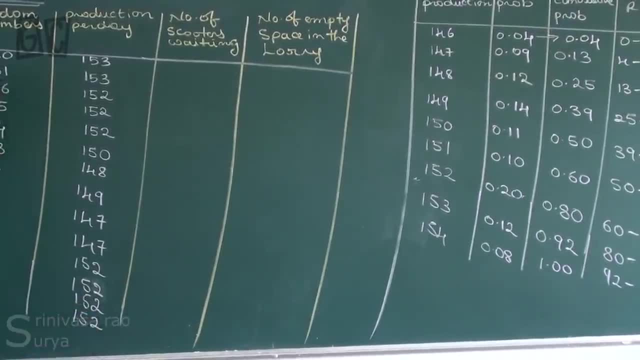 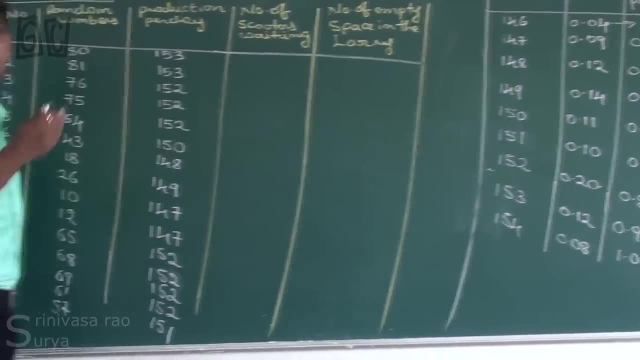 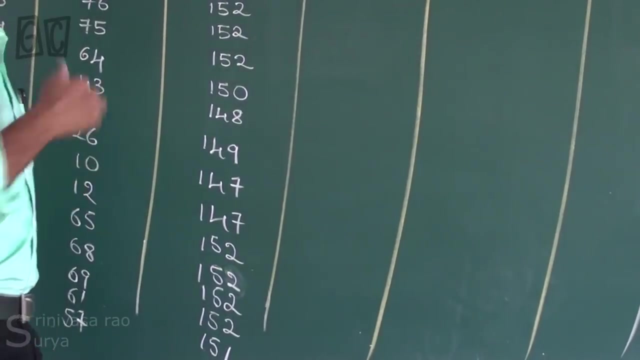 61, again 152. And finally, 57 is right, between 50 to 59, that is 150.. This is our production per day as per the given random numbers. Now we will remember the number of scooters waiting. So the capacity of the lorry is 150. is the capacity. 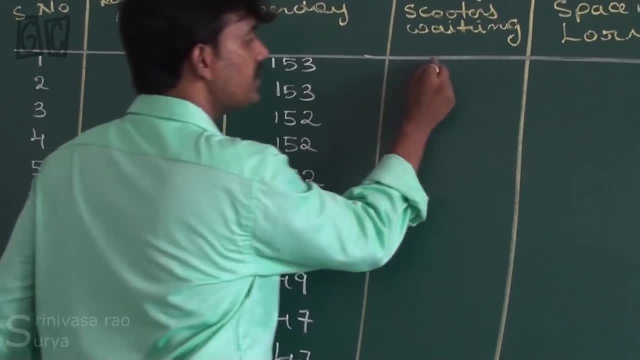 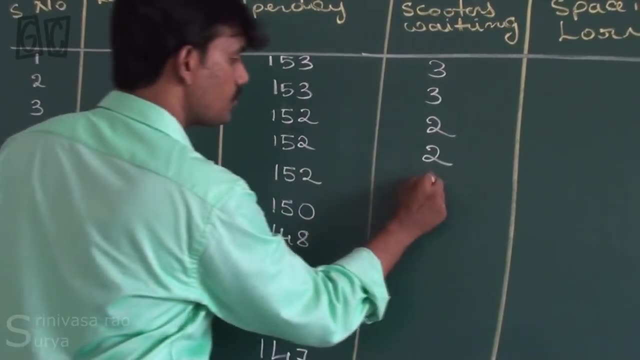 So here, 153 is there. so 3 scooters are waiting right Here, 3 scooters are waiting Here, 2 scooters, again 2 scooters, again 2 scooters, again empty. This I will put an empty. 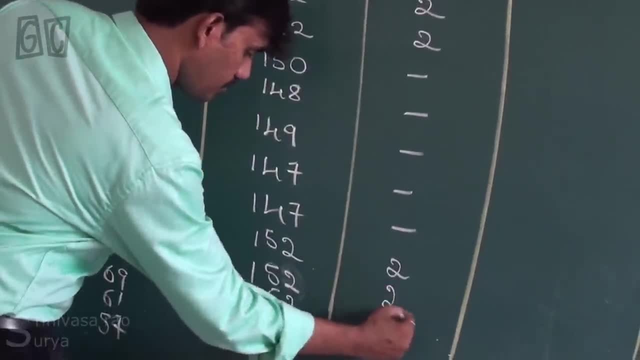 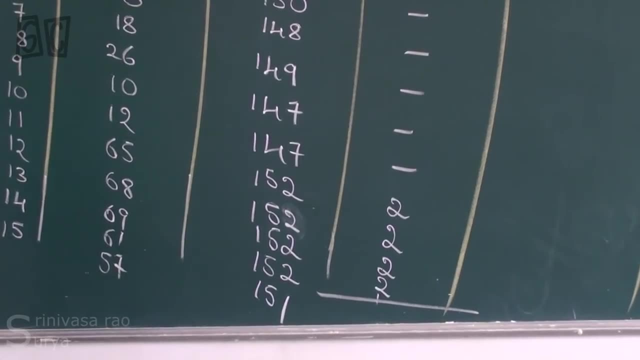 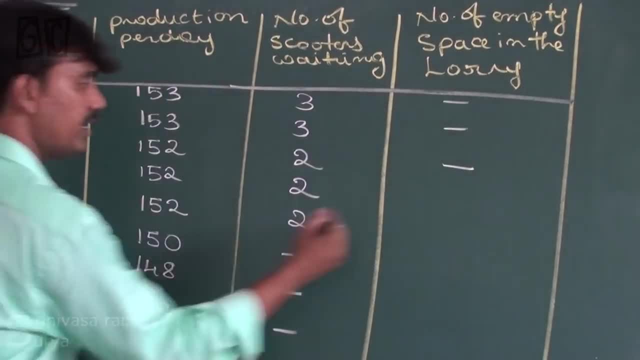 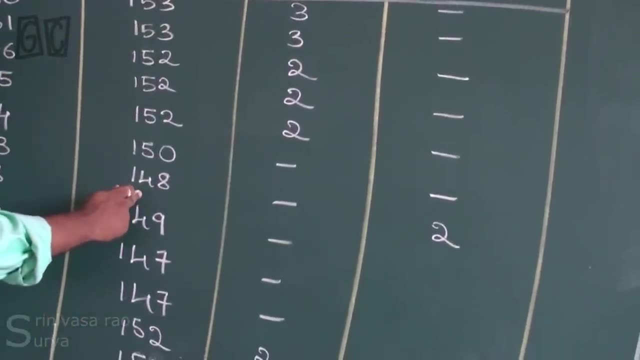 The empty space we don't have, we don't have. again we don't have. Why? because all the values are greater than 1.. Here we have 2 empty spaces. Why? because 148,. the capacity of lorry is 150..